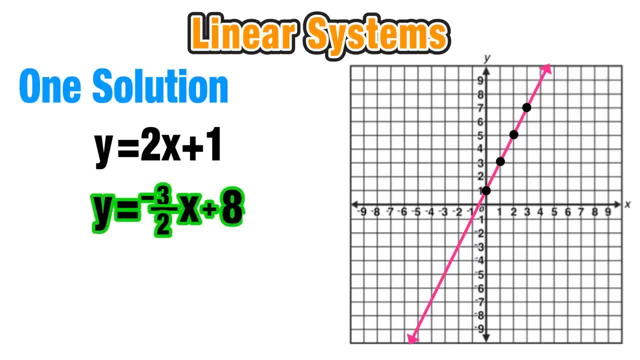 using the slope to construct the line equals negative 3 over 2 x plus 8, that's in mx plus b form. So again I start at the y intercept and graph the line. Now that intersection point with coordinates at is our one. 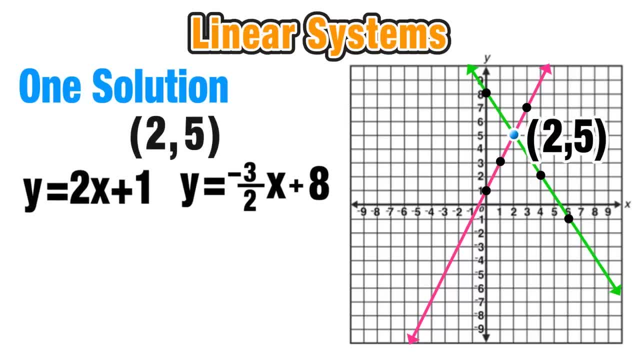 and only solution to this linear system, And we can go ahead and quickly verify this algebraically Using the coordinates of the solution at. we're going to substitute x and y for those x coordinates and y coordinates. So we'll replace the x's with 2's and the y's with 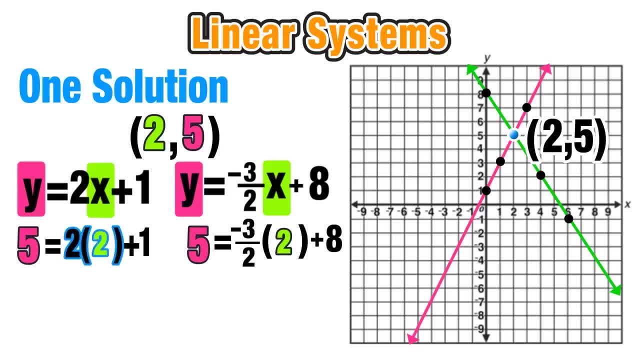 5's and then go ahead and solve and see if this checks out. So for the first equation, 2 times 2 is just 4, and then I add 1 to that, so 5 equals 4 plus 1, of course equals 5.. 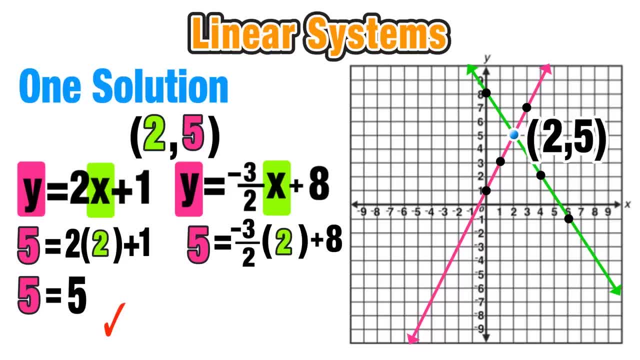 So the first equation checks out because 5 equals 5.. Now the equation on the right: negative 3 over 2 times 2 equals negative 3. Adding 8 to that negative 3 plus 8 does equal positive 5.. 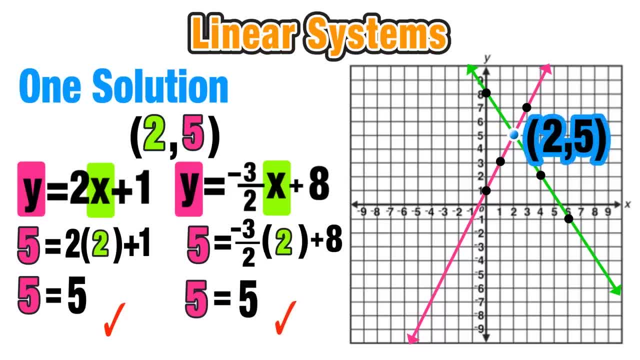 So that also checks out. Now, 2 times 5 is the only solution, is the only point that will work for both of these linear equations. You can try any other point. it might work for one, but it will not work for both. Go ahead, I dare you, try any other point, do it. 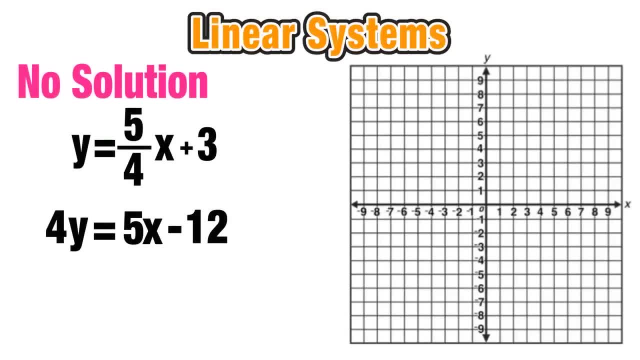 So now, what's the deal when there's no solution to a linear system? Now the first equation is in mx plus b form, so I'm ready to graph it. I start with the y intercept, use the slope and graph the line. So we're good on the first line. Now notice that the second 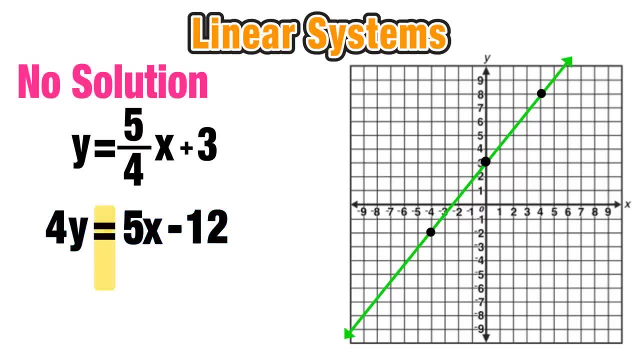 line is not in y equals mx plus b form. I have to get rid of that 4 attached to the y on the left side. The opposite of multiplication is division. So by dividing everything by 4 I cancel out the 4 on the left side. 5 divided by 4 I'm going to leave as 5 over 4 because 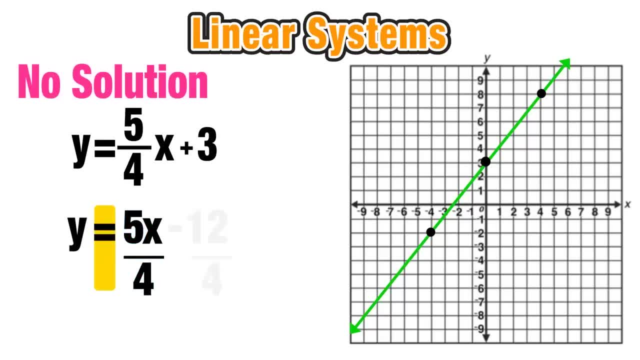 it can't be simplified. Negative 12 divided by 4 is negative 3. and now my line is in mx plus b form and I can graph it. Notice here that these two lines have the same slope: positive 5 over 4.. That means that